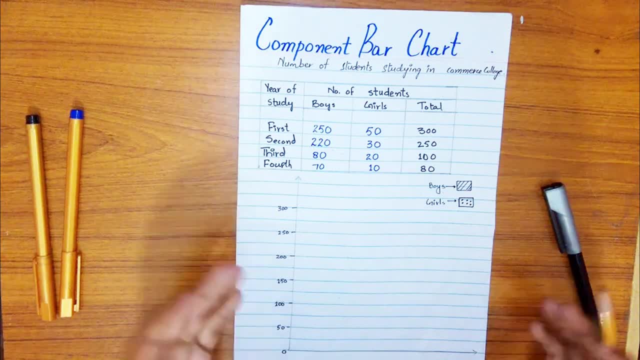 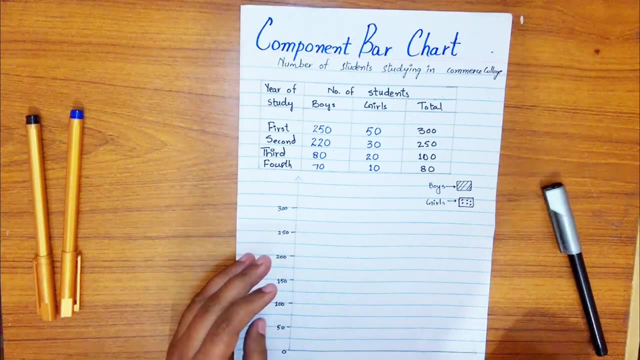 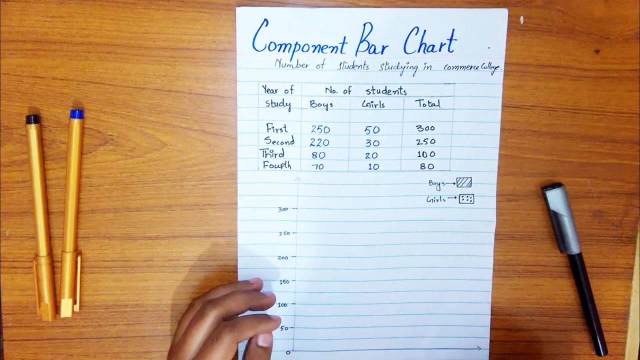 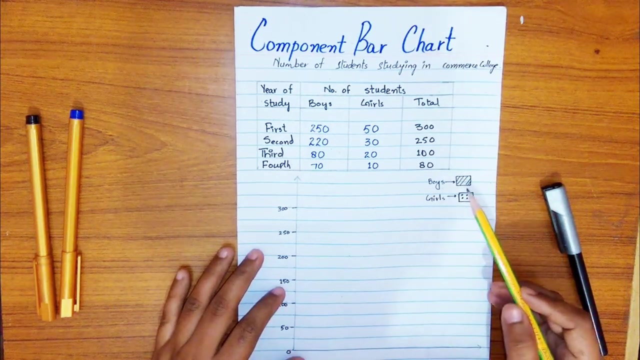 For drawing it. we make simple bars representing each component over one another. The total of all components represent the total length of each bar. In order to distinguish the various components of each bar, we use different colors or different patterns, Just like I made two patterns here for boys, this, for girls, this. 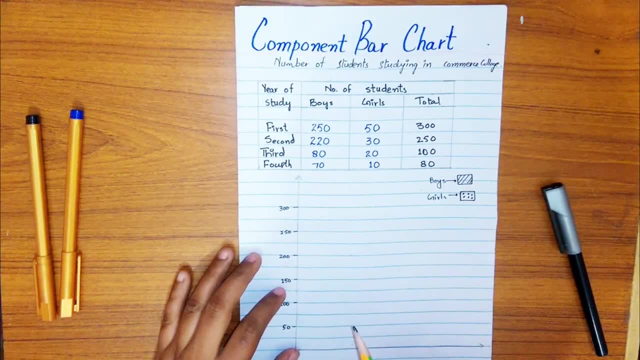 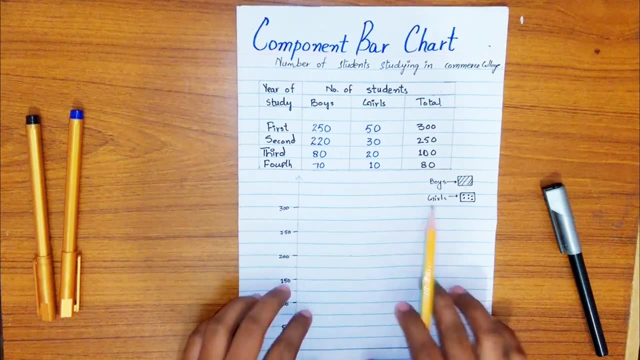 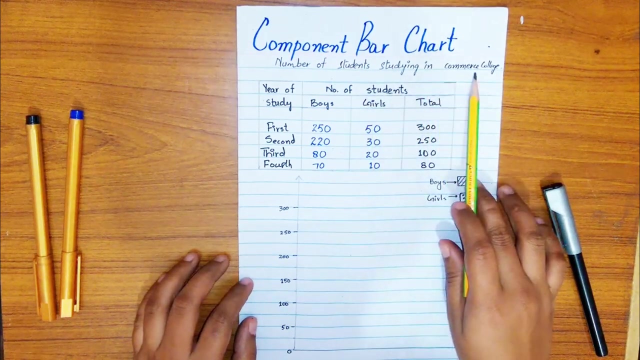 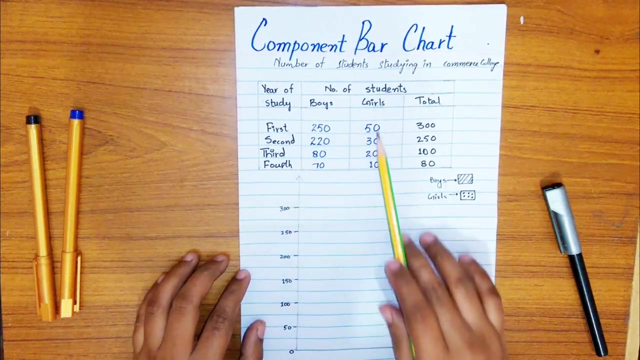 The component bar chart may also be represented by the percentage. Here we are going to construct a simple component bar chart. I have a data set of number of students studying in commerce college, The number of boys in different era of studies and the number of girls in different era of studies and total number of students. 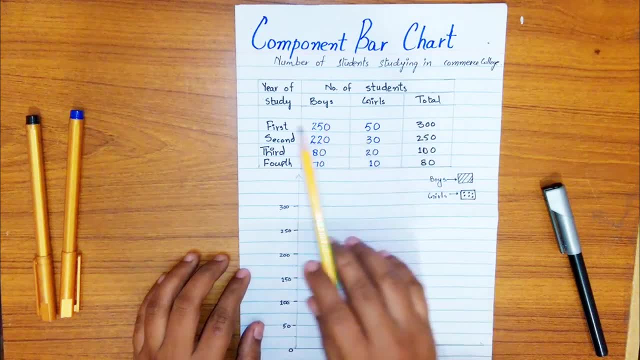 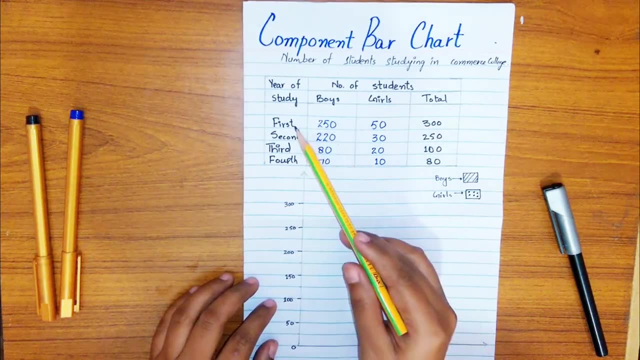 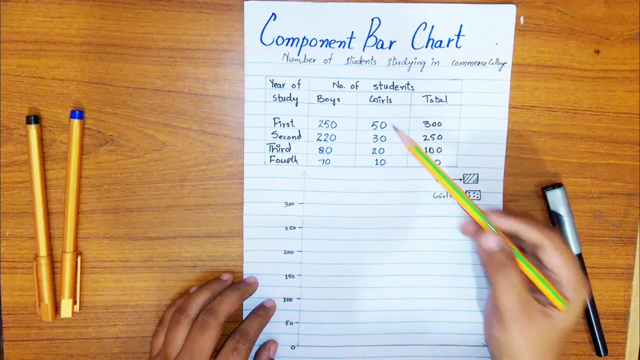 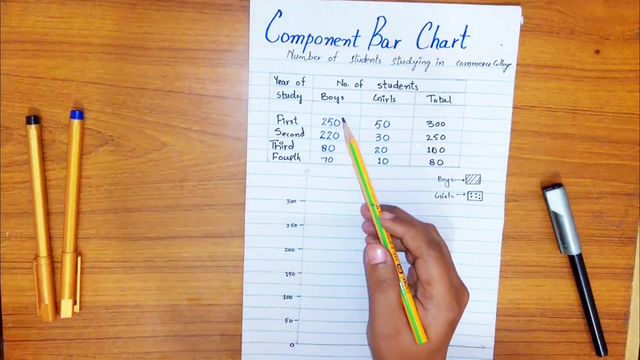 Now we construct component bar chart with the help of given data set. First of all, we make bar charts for first year, second year, third year, fourth year- boys. Then we will construct a bar for girls. In first year there are 250 boys. 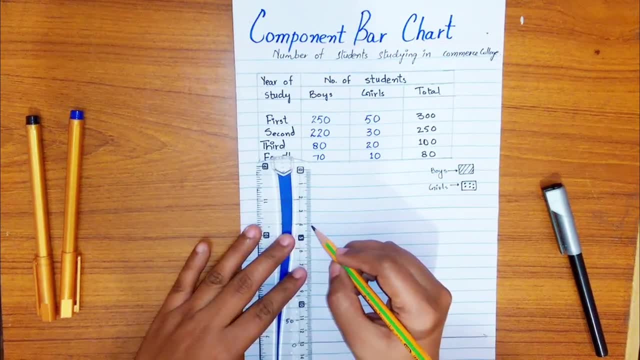 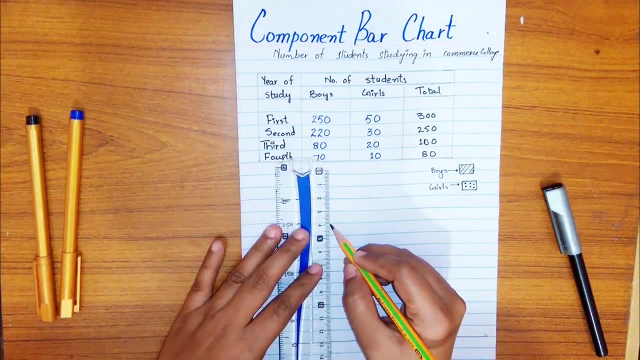 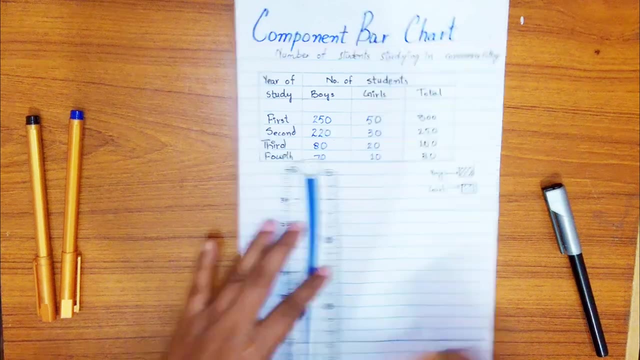 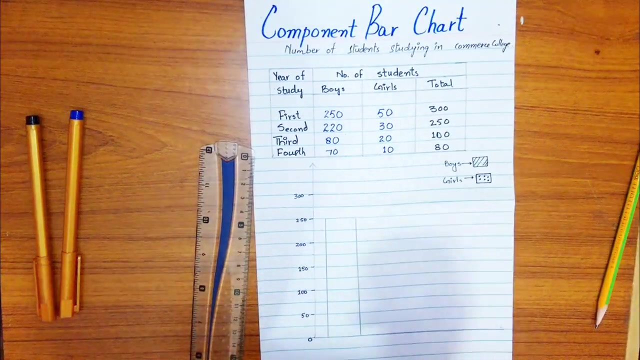 250: 20, 21, 22, 23, 24, 25, 26, 27, 28, 29, 31, 32, 33, 34, 35, 36, 37, 38, 39, 41, 42, 43, 44, 44, 45. 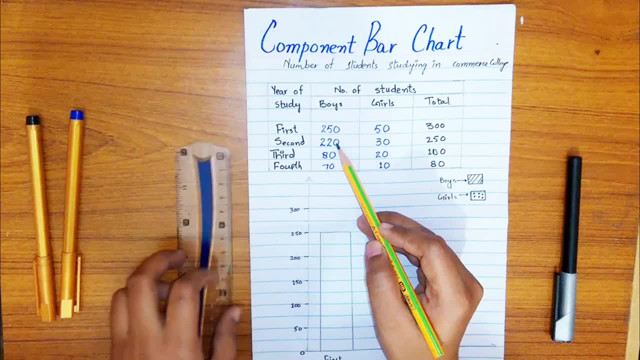 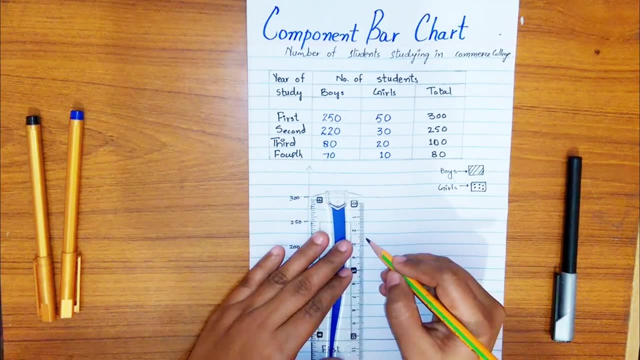 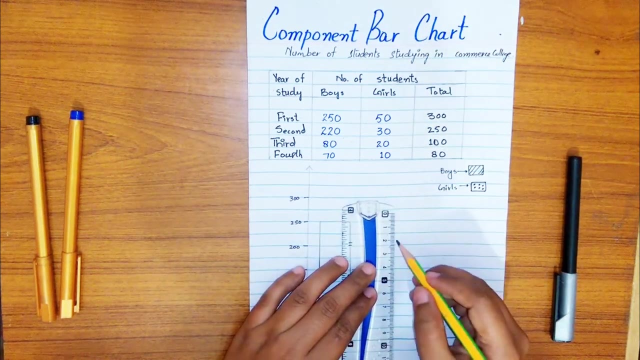 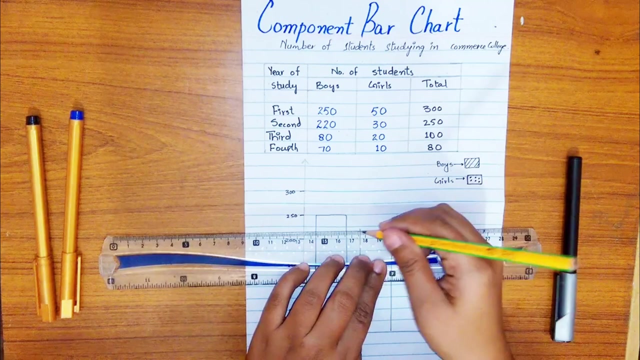 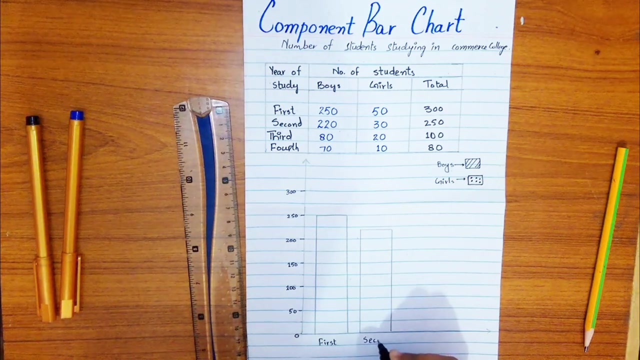 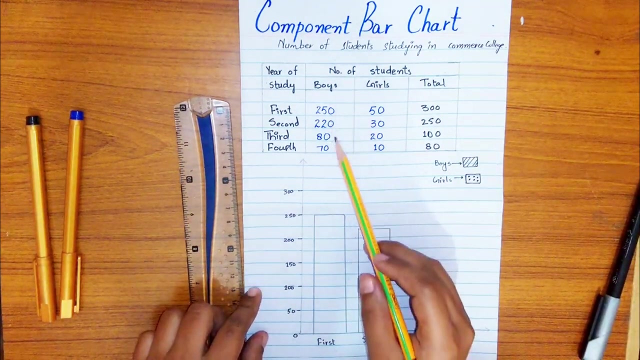 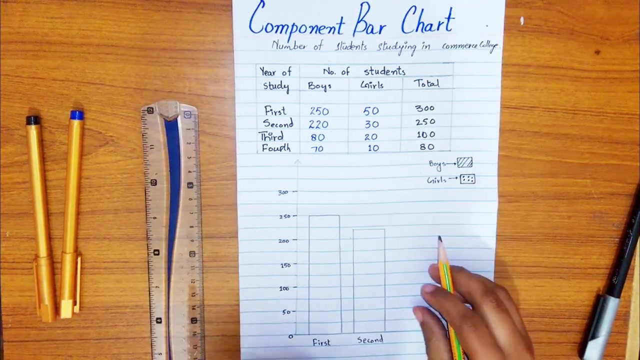 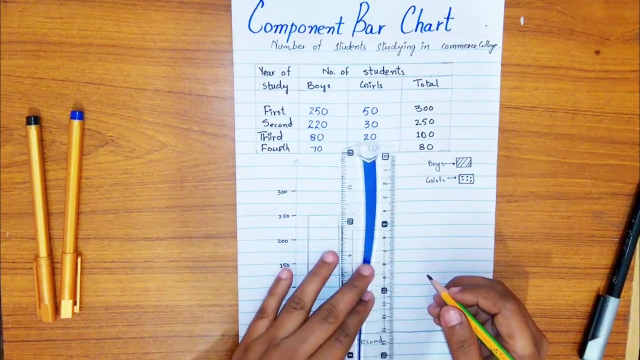 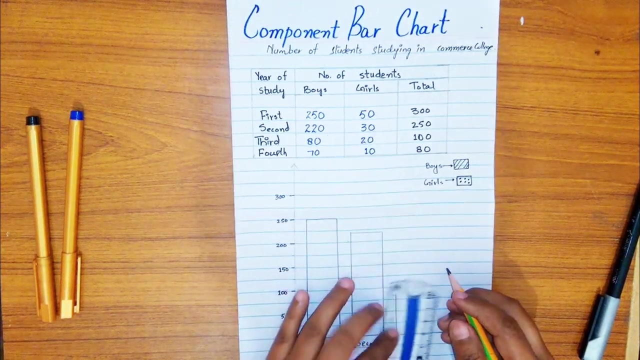 45, 46, 46. two hundred and twenty boys. two hundred and twenty is somewhere here. we have 80 wise in the third year. 80 is somewhere here, sorry, it's somewhere here. make sure the width of the circle is equal to the width of the circle. we have 80 boys in the third year. 80 is somewhere here, sorry, it's somewhere here. make sure the width of. 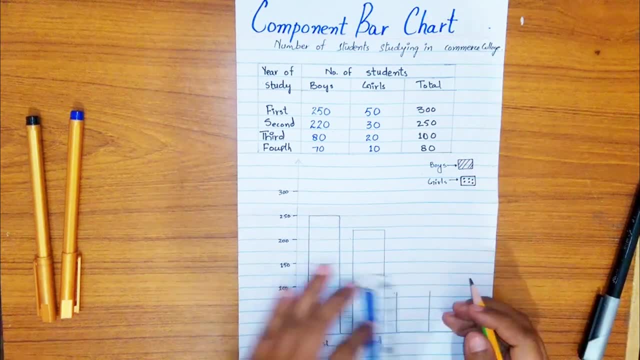 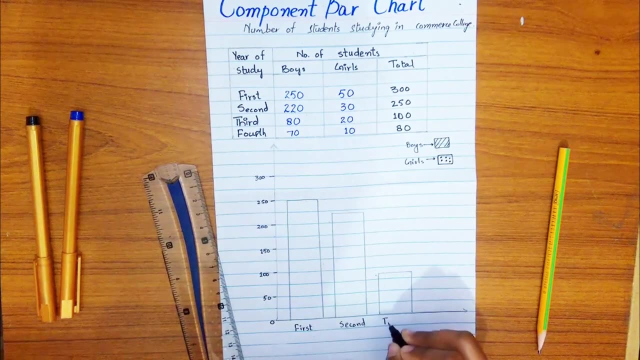 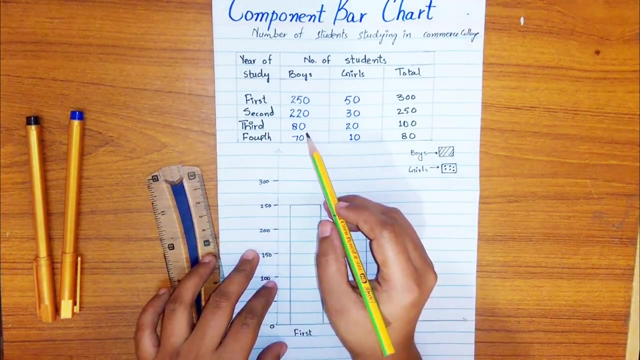 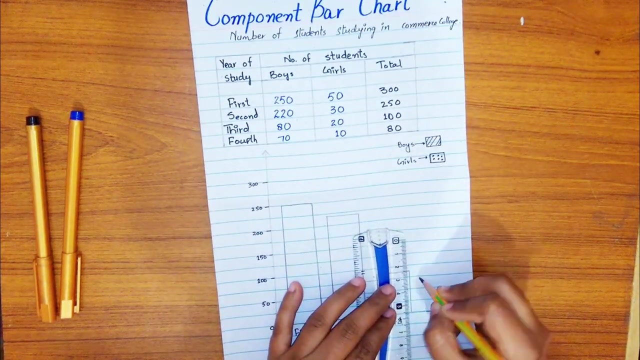 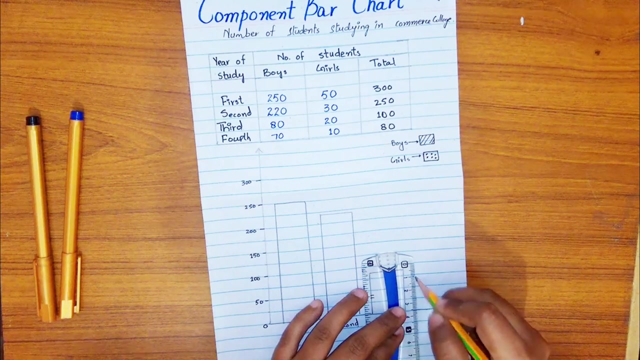 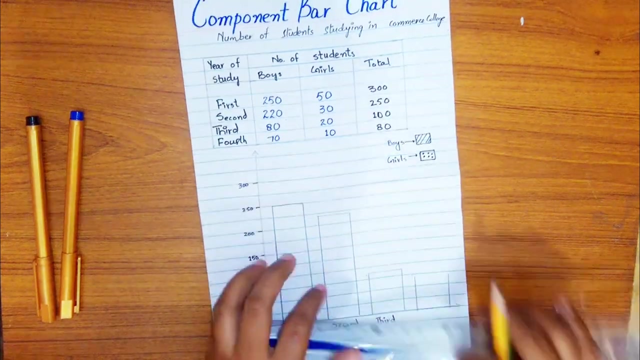 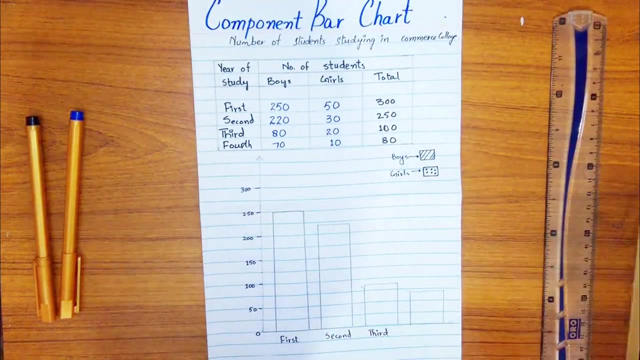 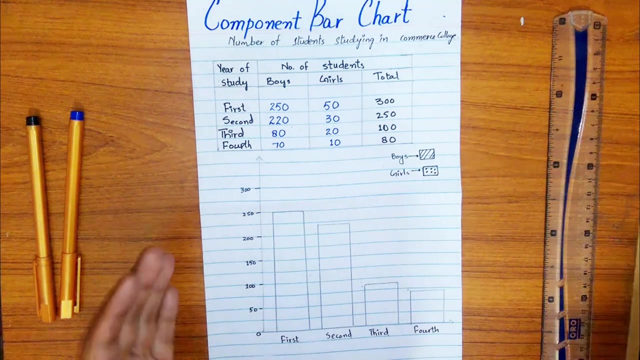 all the bars is equal. here we have third year and in the fourth year the students in Commerce College which are wise are 70- 70 is somewhere here. we have 80 boys in the fourth year- 80 is somewhere here. here I have drawn all the bars for boys, which is our first component. here I have 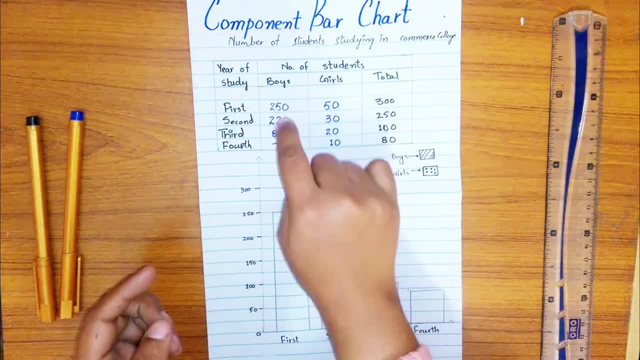 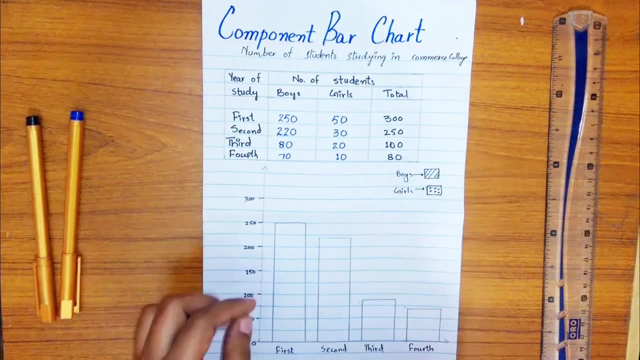 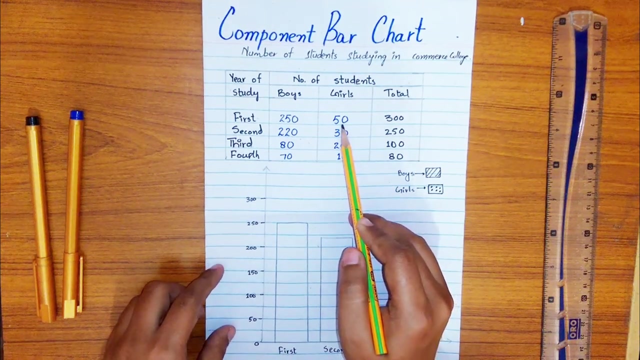 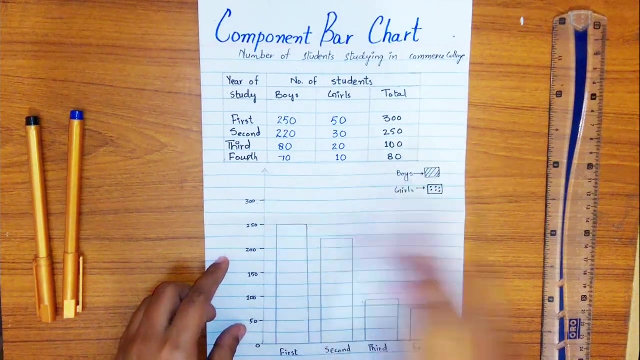 drawn all the bars for boys, which is our first component. now we are going to construct a bars for second component, which are girls. now how many girls are there in first year? 50 to 250 plus 300. 250 plus 50 is equals to 300. 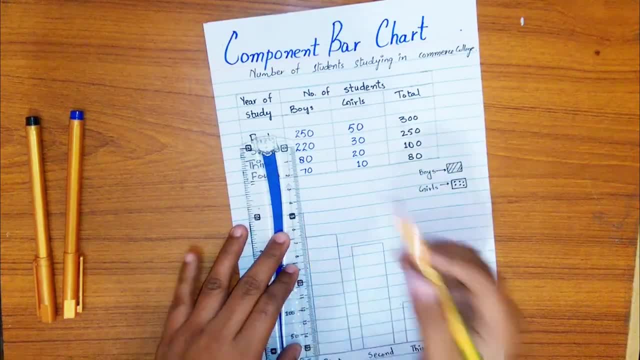 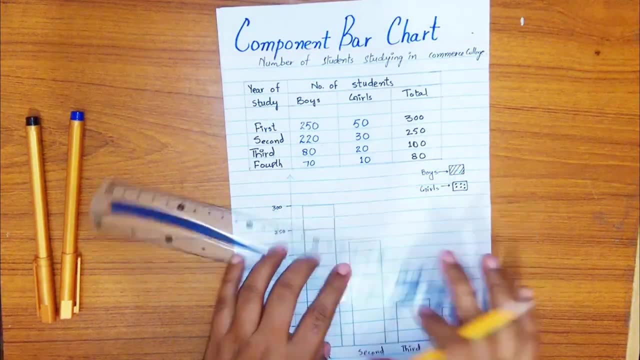 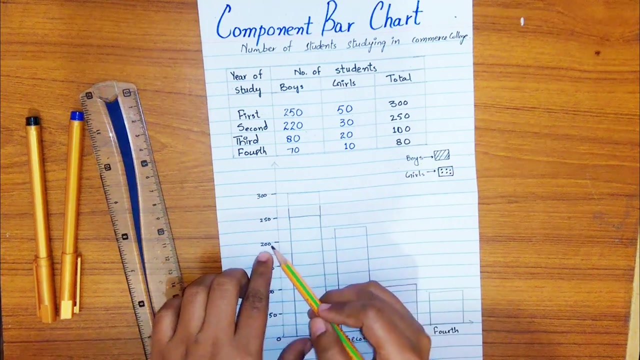 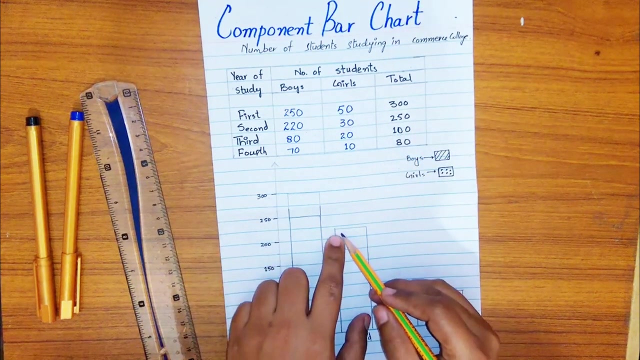 no, now the girls studying in second year are 30. 200 plus 30 is sorry. 220 plus 30 is equals to 250. here I have made a bar for boys, we which are 220 in second day. now I am going to make a bar for boys which are 220 in second day. now I am going to make a bar for boys which are 220 in second day. now I am going to. 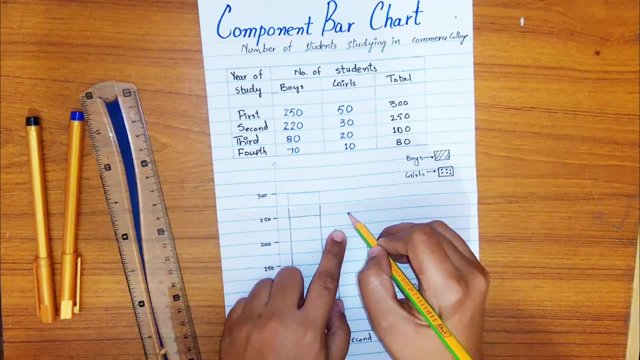 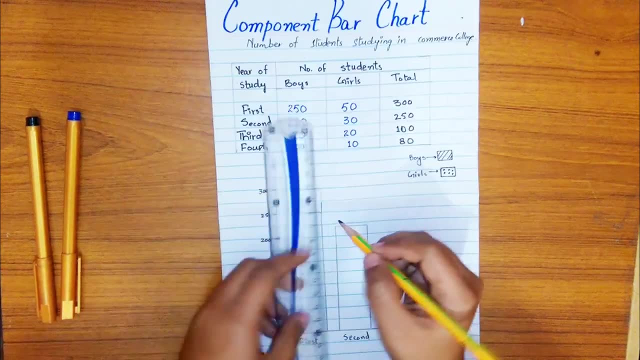 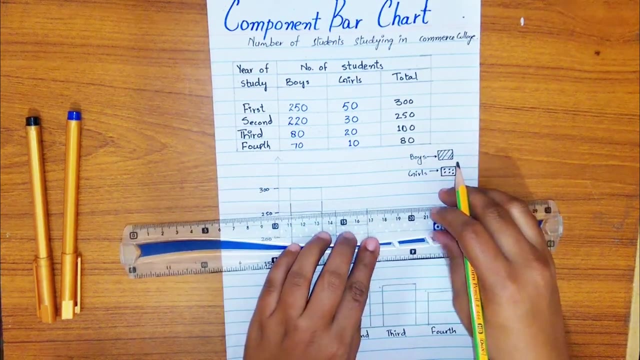 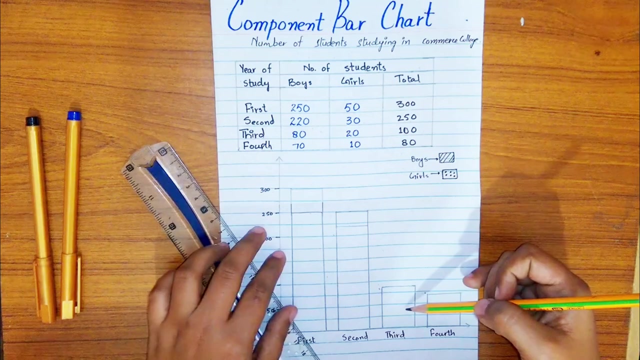 construct a bar on over it for girls which are 32, 20 plus 30, which is equals to 250. 250 is here. we just expand our bar. now for same for third year. only 20 girls are studying in third year and the total of 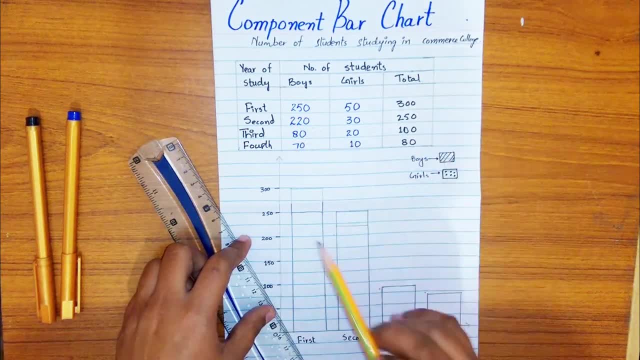 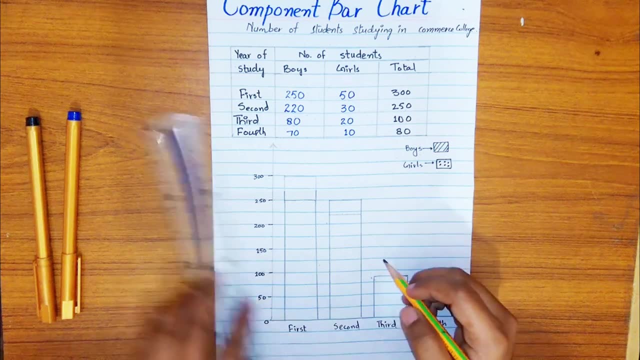 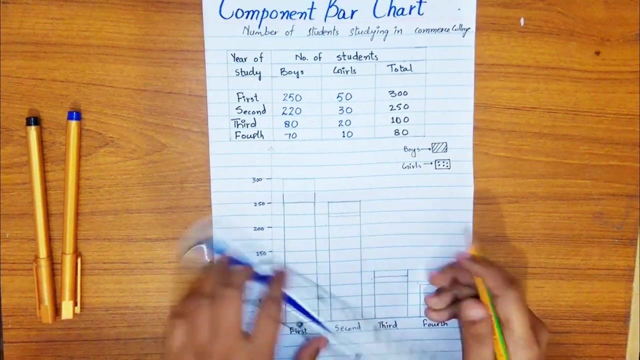 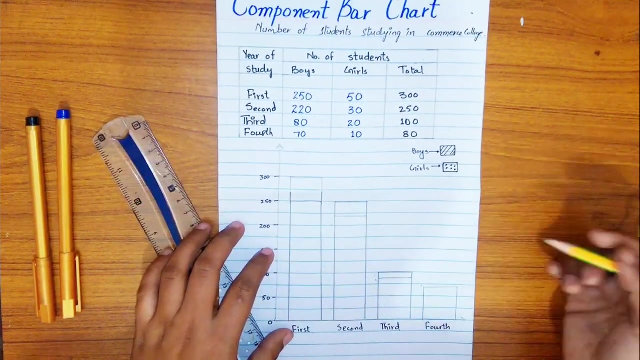 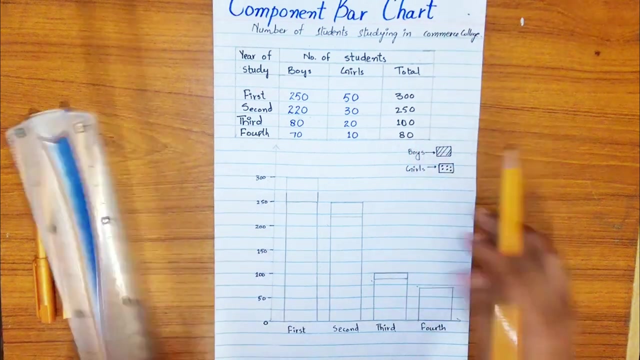 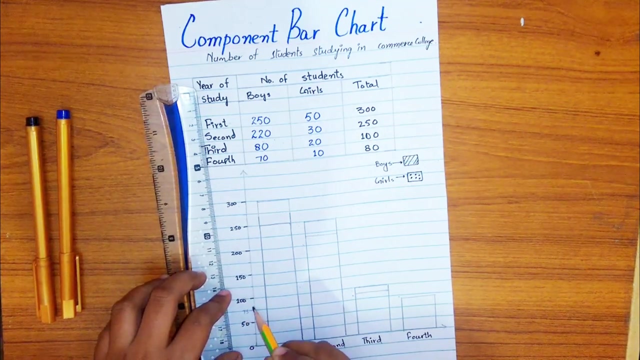 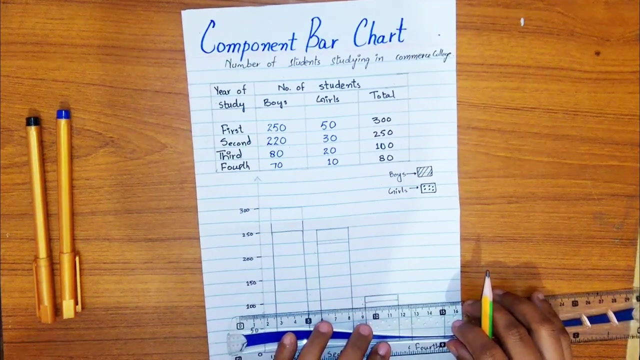 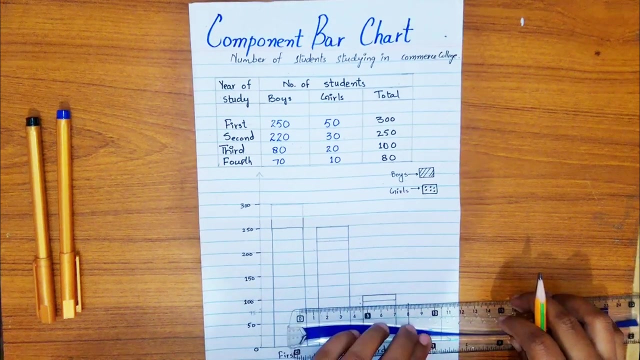 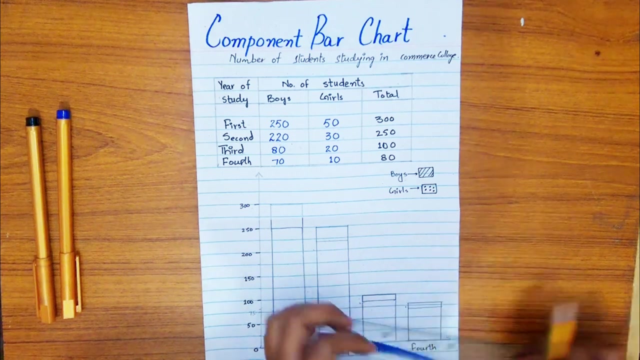 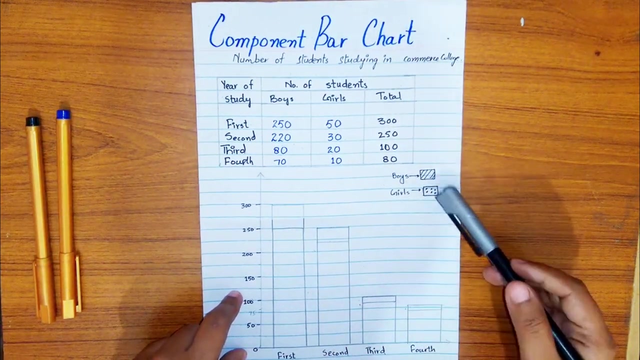 80 boys and 20 girls, which is equals to hundred number of students. here we have already construct a bar for wise. now for girls. in fourth year there are only 10 girls, which makes the sum of 80. 80 is somewhere here. now for showing the differences between these bars, I have made pattern here for 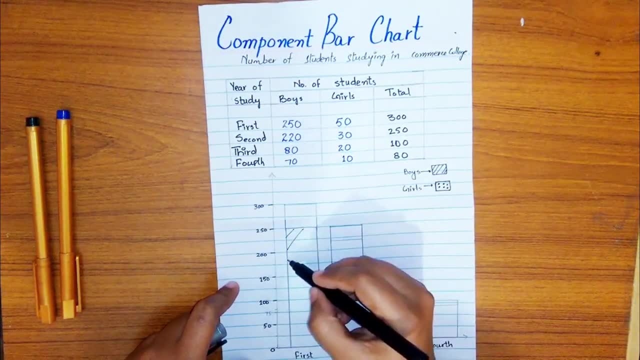 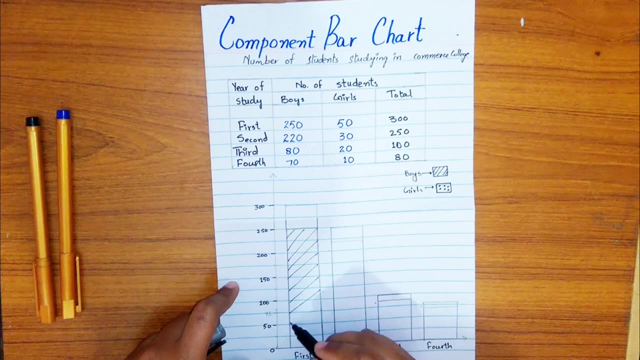 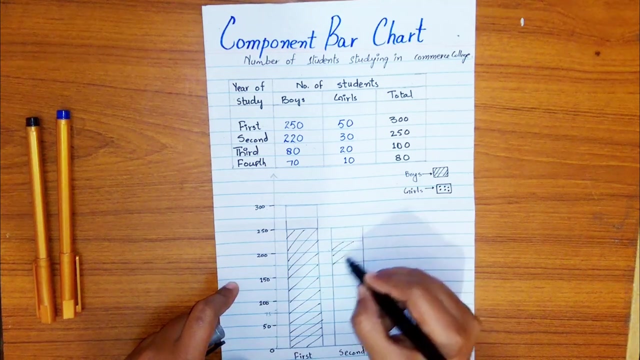 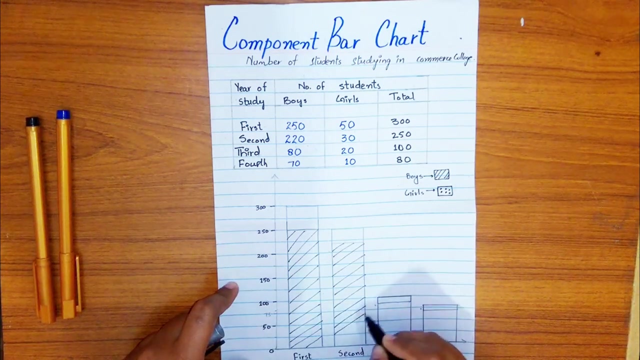 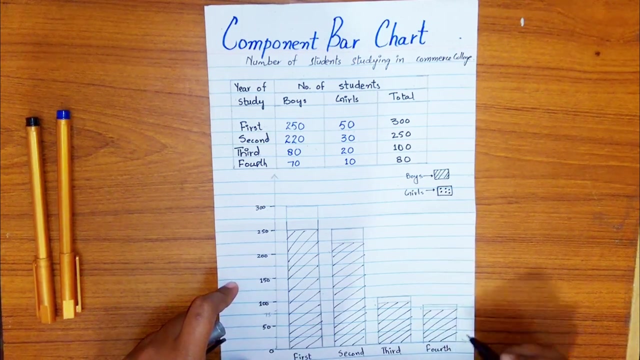 boys. draw a line like these so we can differentiate who are the boys and who are the girls. do the same for all. you can also draw pattern only on second bar of second component, not on first component. so it also shows that blank is for boys and the pattern is for girls. but here I